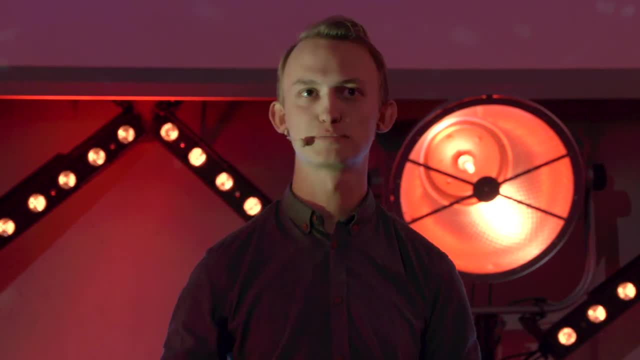 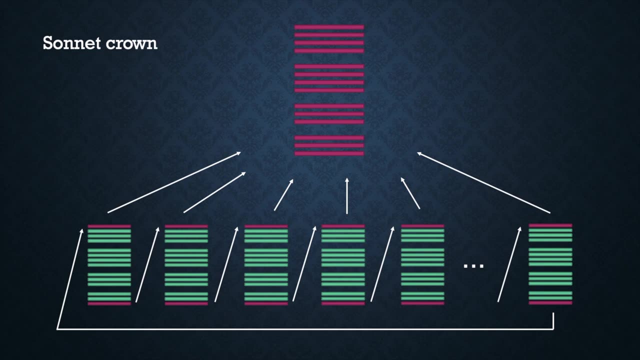 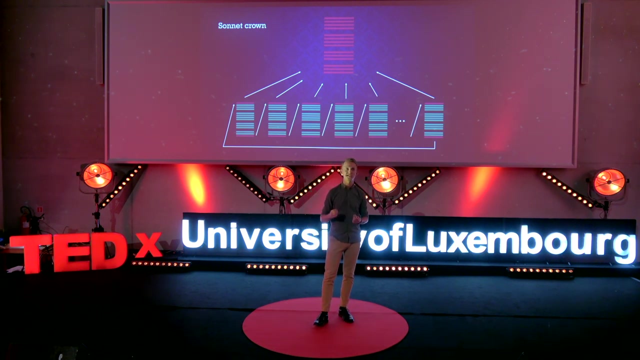 circle. you take the last line of the last poem and set it to be the same as the first line of the first poem, forming a circle or crown of sonnets. Now, if done correctly, a 15th sonnet emerges, consisting of the first lines of each. 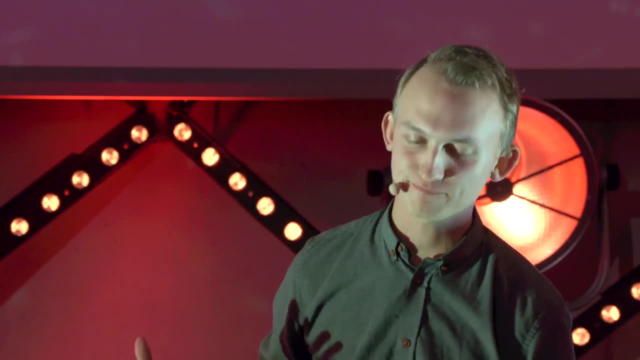 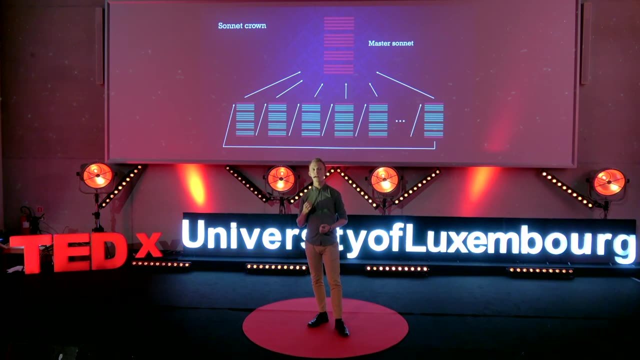 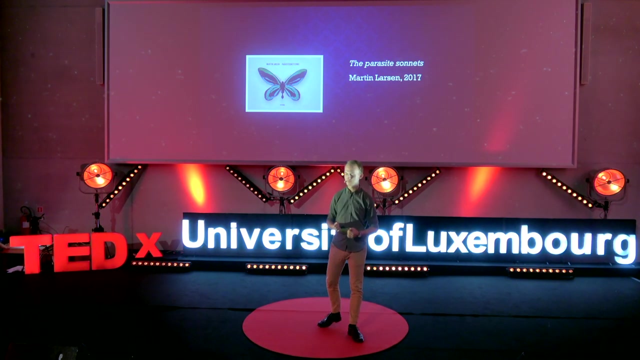 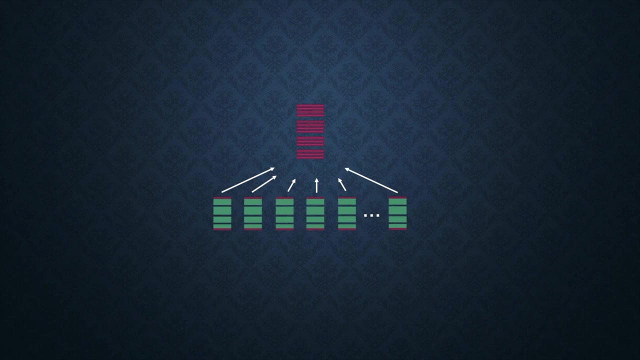 sonnet. This is the master sonnet. Now. this is a very systematic way of writing poetry, with a very heavy structure, An intriguing structure. Two years ago, the Danish author Martin Larsen asks in the parasite sonnets: if 14 sonnets combine to form one Master Sonnet, then 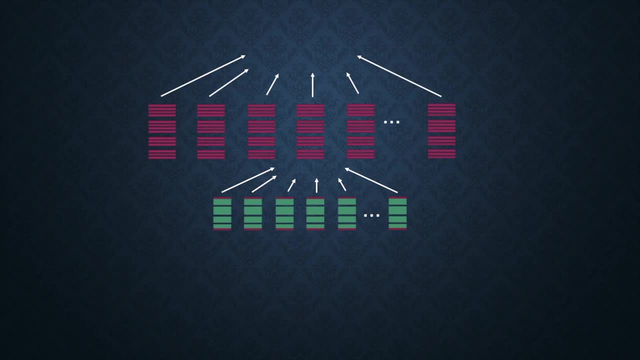 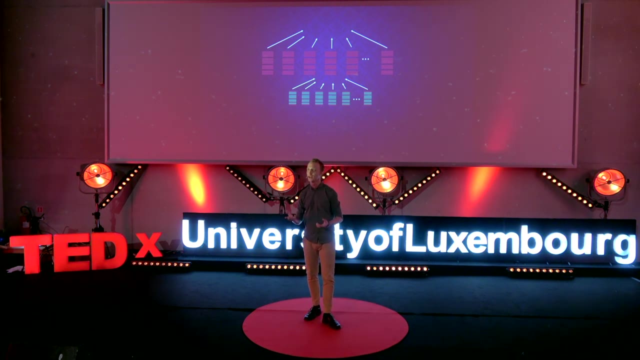 14 such Master Sonnets could also combine to form an even higher master sonnet, A master of masters. And what if that was already the case? What if each of our sonnets was a master containing 14 poems? then you have something interesting. 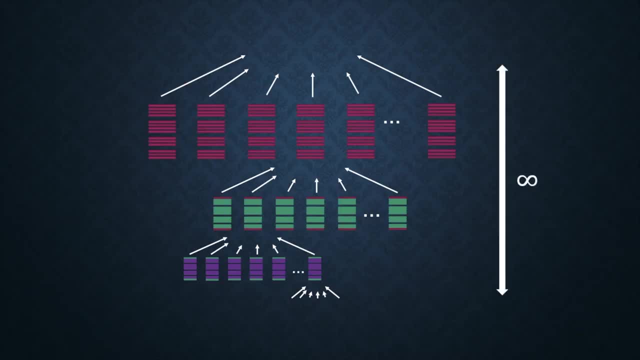 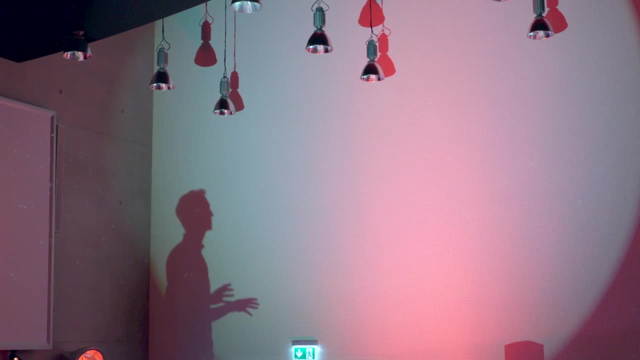 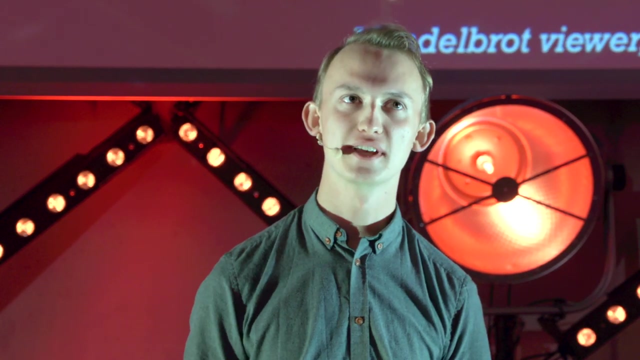 Then you have an infinite structure of poems within poems, rhyme schemes weaving through each other. Larsen calls it fractal poetry. Now, you may know that the special thing about fractals is that, no matter how much you zoom in on one of the edges, 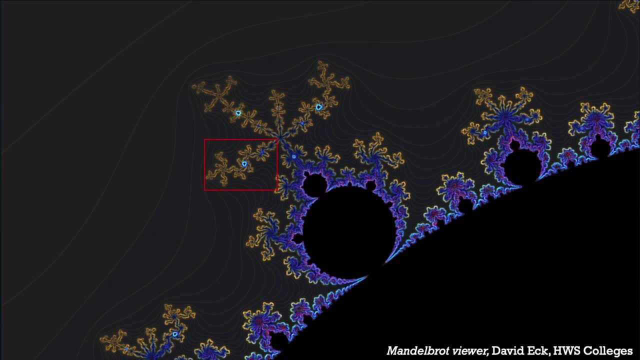 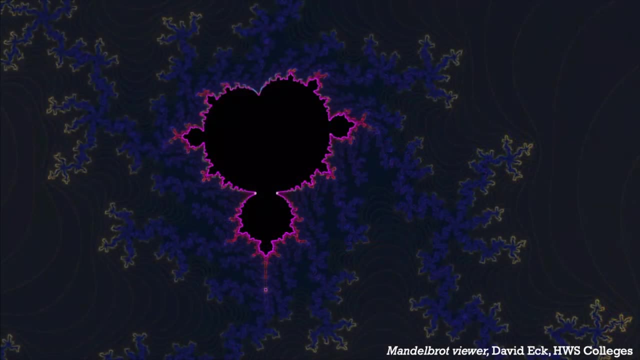 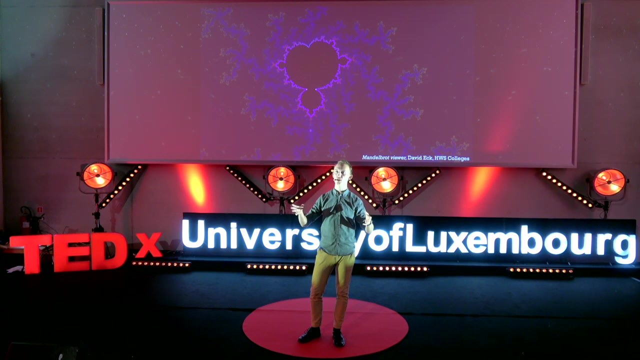 it remains infinitely detailed, intricate and self-replicating. In the same way, we can zoom in on our sonnet crowns and see them expand into more and more poems, or we can zoom out and see the poems contract into masters. 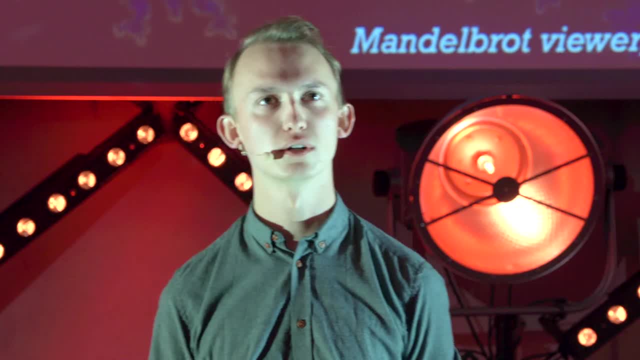 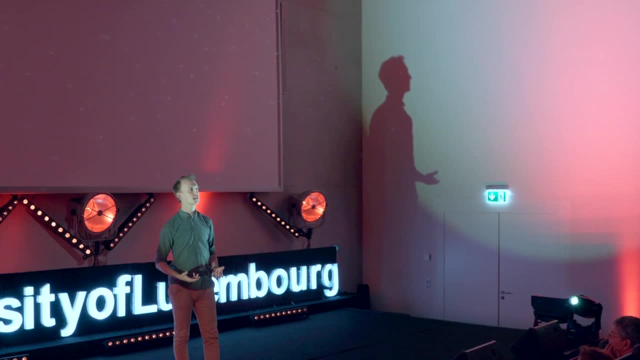 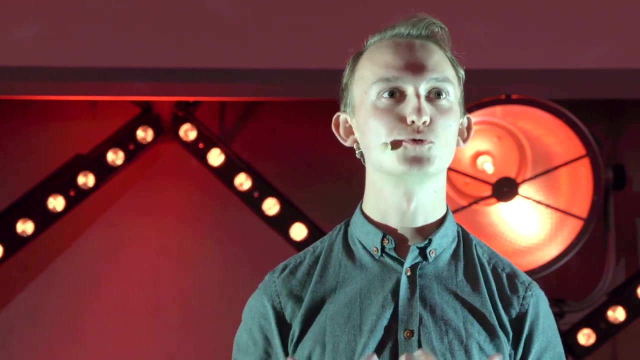 giving us this fractal poetry. But there is more here than just geometry, Because poetry is about words and what those words do to us. So to fully explore this fractal poetry, we need to write poetry. We need to write a lot of poetry really fast. 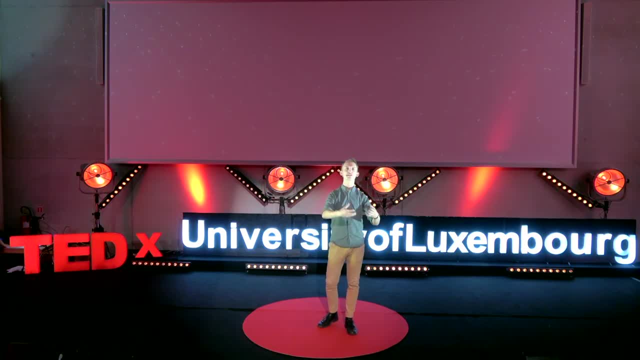 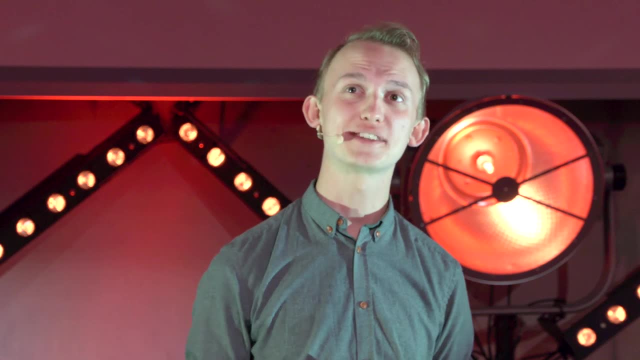 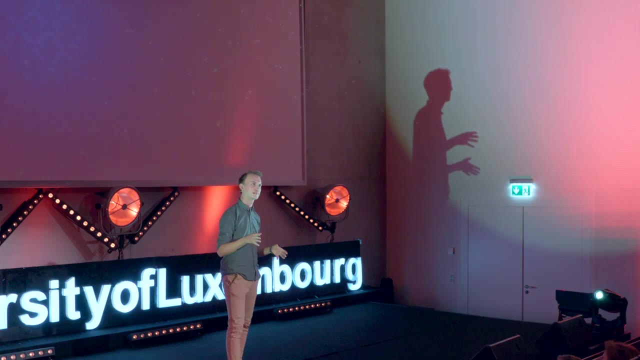 so that wherever we go in this structure, there's always more poetry to be found. This is not really something we can do, but we can make the machine help. To do that, we need to make a computer solve three tasks. First, we need to make it write a line of coherent text. 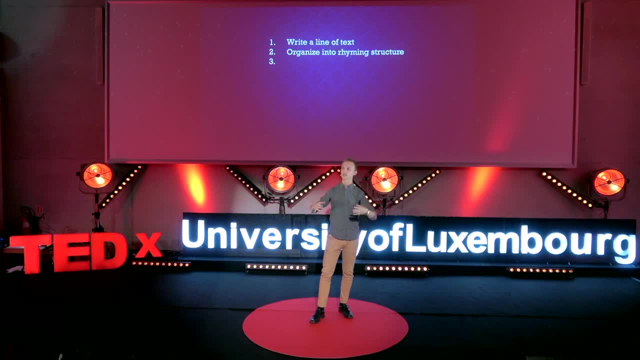 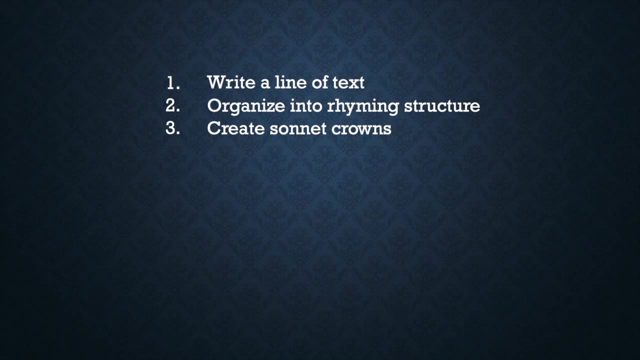 Then we need it to put these lines together in a rhyming structure And finally we need it to combine these rhyming structures into sonnet crowns that we can create our fractal poetry with. Now, writing coherent text which is rhyming is really hard. 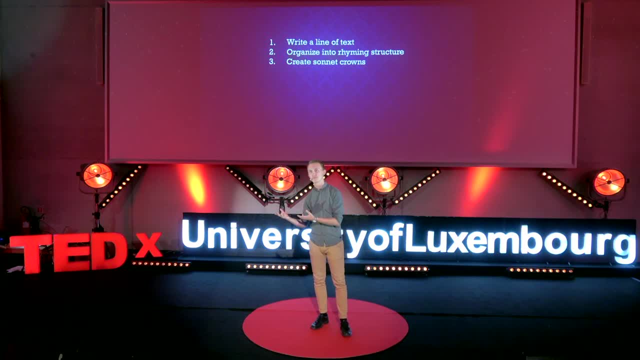 Also for a computer. Luckily, there's already code written which can help us with the first two of these tasks. A module named Markovify can help us solve the first task. You feed it a pile of texts like the collected works of Sherlock Holmes. 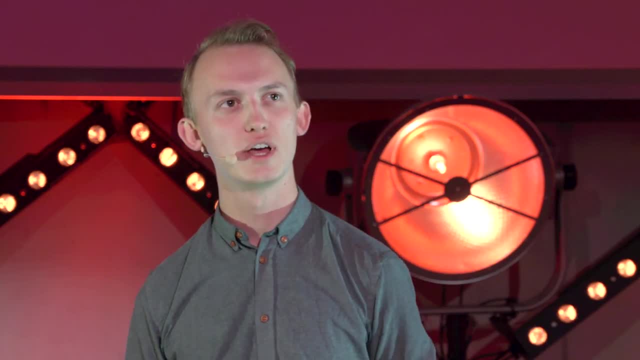 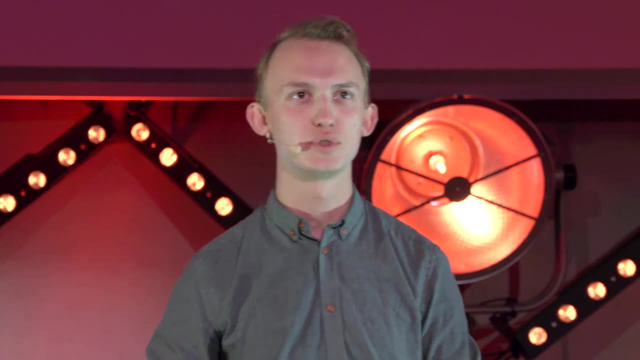 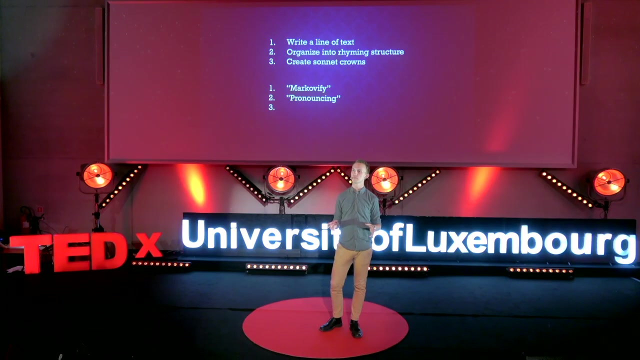 And then it uses a very simple statistical process, called a Markov process, to use these texts and combine it into new sentences, which are mostly coherent. Using another module named Pronouncing, we can even make it rhyme, And since machines are so good at structure, 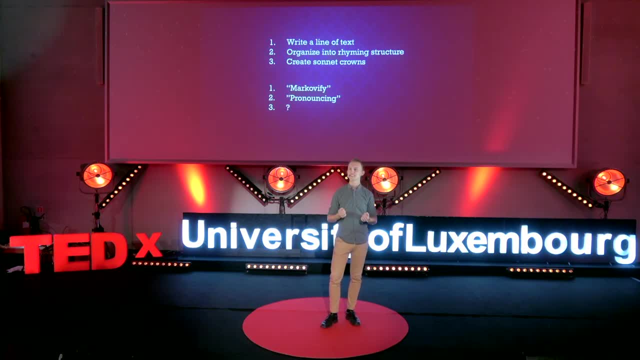 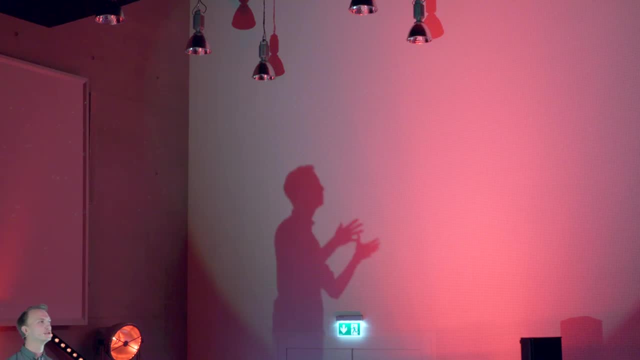 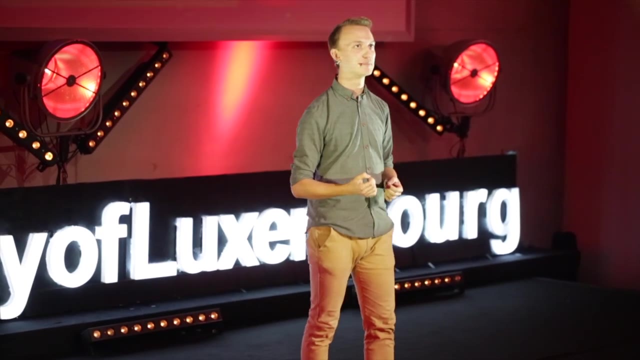 in many ways. the last point is the easy one, But it is also the most important one, because that is what makes what we are doing into something new, something not done before. A friend of mine is a brilliant linguist, and by teaming up with him, 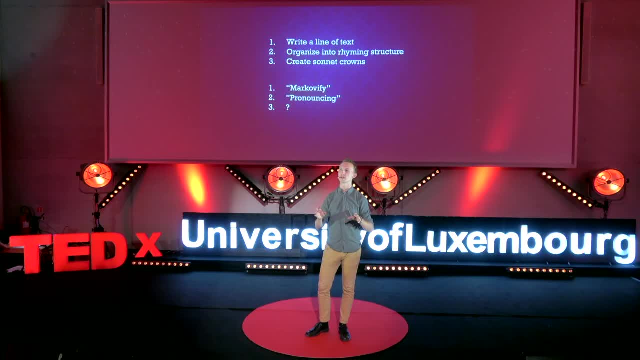 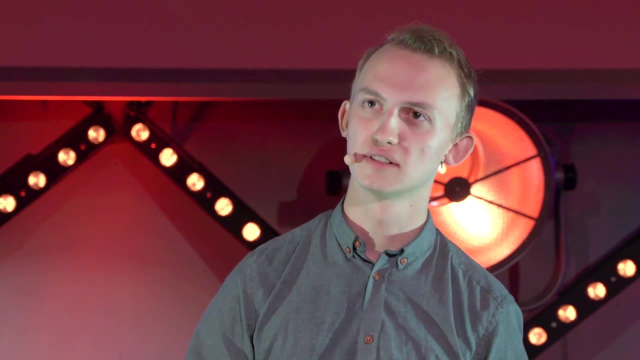 we actually managed to solve this with comparably little programming. So much had already been done. we just needed to twist it in our own way, And so let us look at what the machine can do. For the sake of time, we will look at quartets, not sonnets. 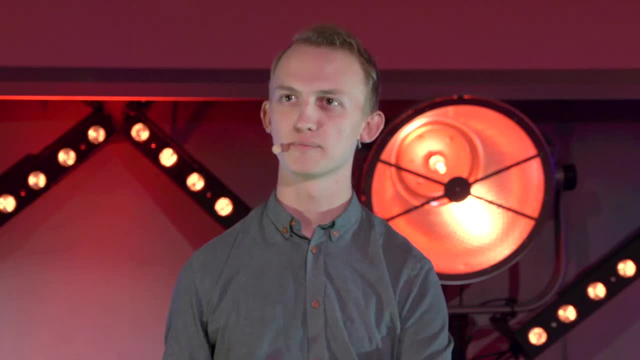 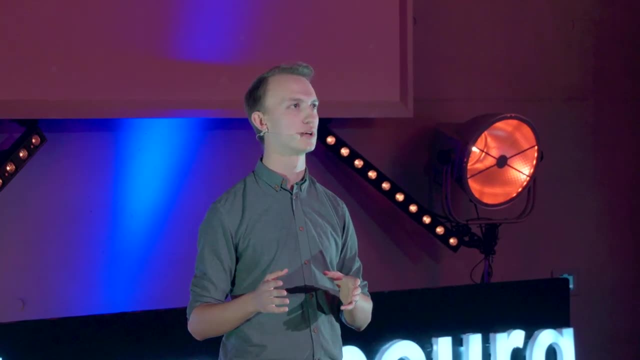 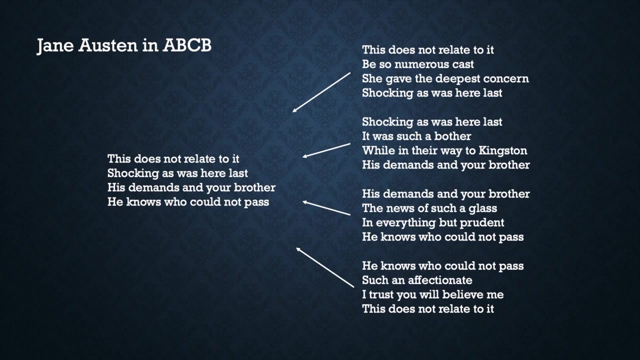 This means that our poems have four lines instead of 14.. So we asked the machine to write poems on an ABCB structure using the works of Jane Austen. This is what we got. So, as you can see on the right, you have the poems. 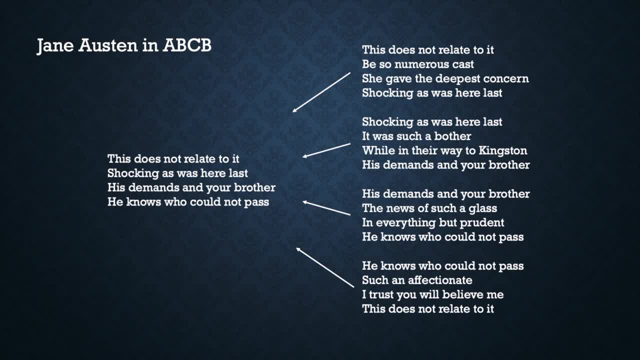 where the last line is used as the first line of the following poem: On the left you have the master quartet. Let's take a look at that. This does not relate to it. shocking, as was here last, His demands and your brother. 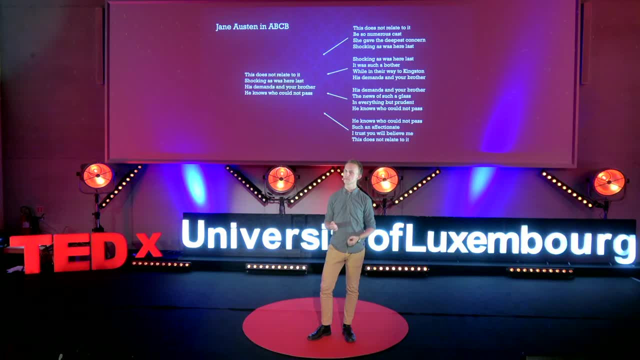 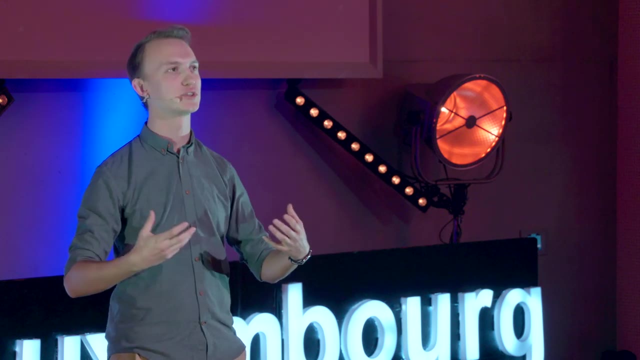 he knows who could not pass. I would dare say that this is not art. It's more like systematic gibberish, And this poem in itself is not interesting, just like a picture of a fractal in itself is not interesting- Only when you start zooming in. 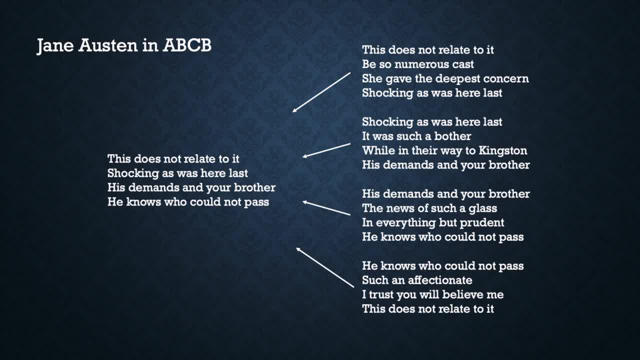 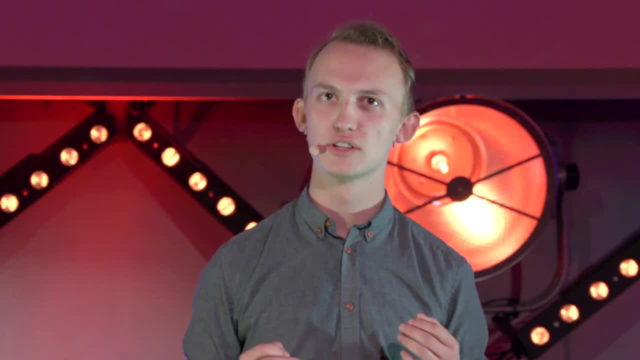 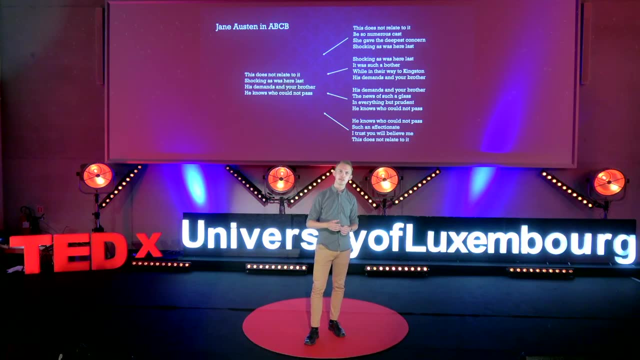 only when you start exploring can you understand the true nature of the structure. Only then does it become something like art. So we need to start exploring this poem. What we can do is we can look at a part of it, say the mention of a road to Kingston. 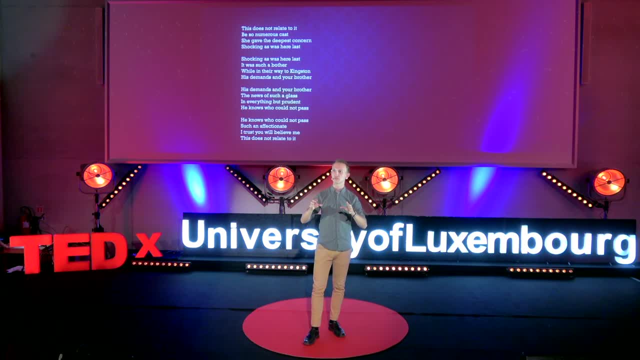 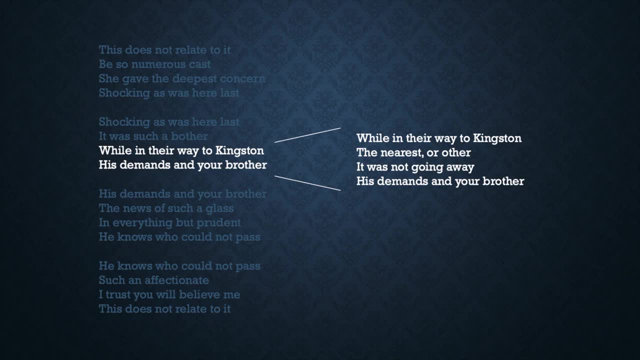 Then we can zoom in on that like we zoom in on a fractal. We let the second poem become the master poem of a new crown And we get the following: While in their way to Kingston- the nearest or other- it was not going away. 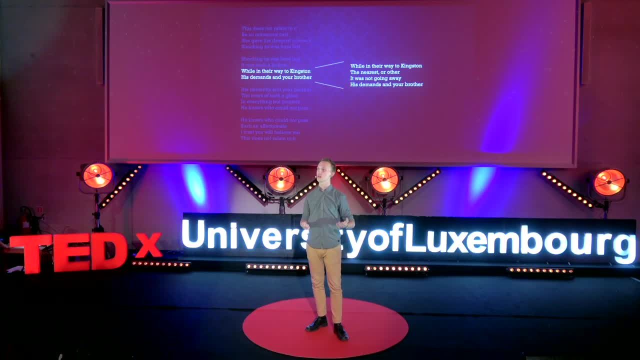 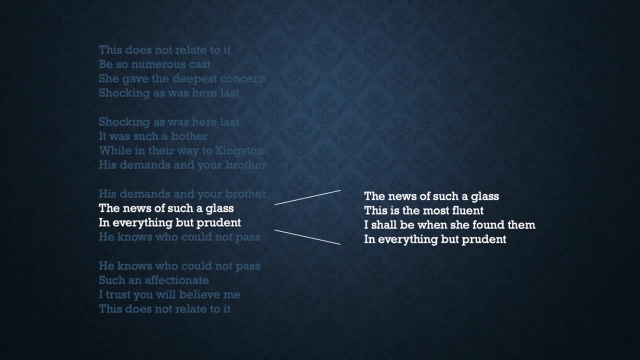 His demands and your brother, Or we could zoom in somewhere else- like we might want to hear about this news of glass, The news of such a glass- this is the most fluent I shall be- when she found them in everything but prudent. 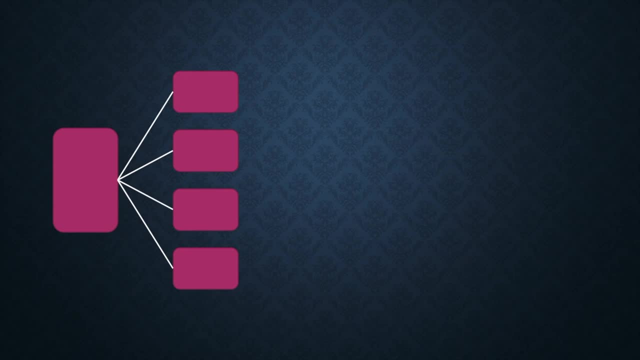 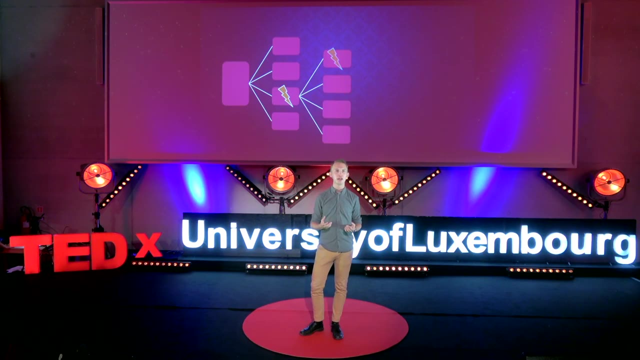 Now, what we are doing here is that we read through an individual sonnet crown until we strike upon something interesting, a poem that sparks our imagination. We then use that poem as the master of a new crown, repeating the process, stringing together a system of interesting words. 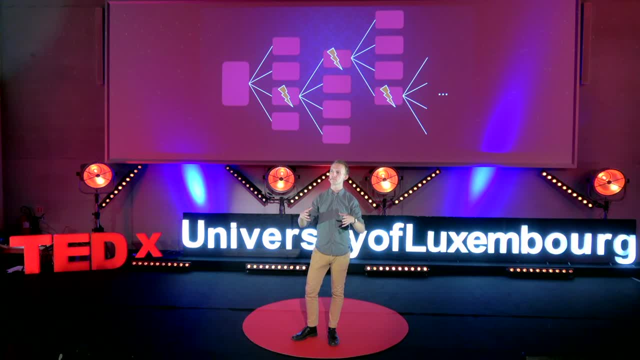 or exploring a theme. We could also go along a more geometric path. For example, we could explore deep along one path of sonnets but then go up along another path of sonnets until we finally return around the loop to our original poem.